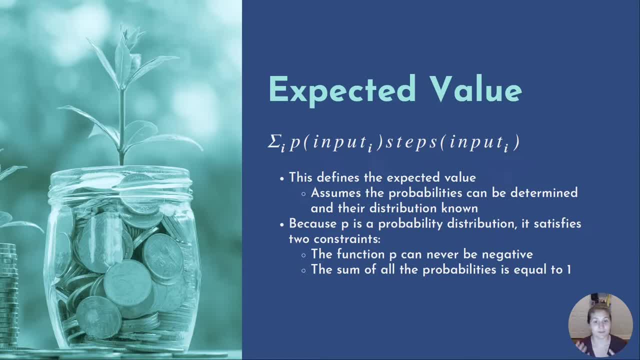 is called expected value. This assumes the possibilities can be determined and the distribution is known. Because p is the probability distribution, it ends up satisfying two constraints: that the function p can never be negative And the sum of all the probabilities should equal one right one hundred percent. Let's look 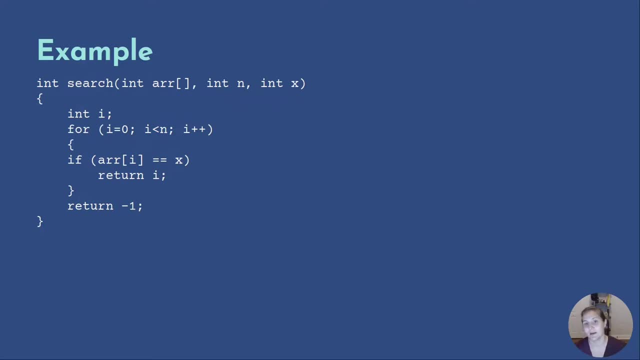 at an example and determine the best, average and worst case of that algorithm. So in the first example we are going to determine the worst case of the algorithm, In this case our algorithm. we are searching within an integer array that is the size of n, Searching through this size and we're trying to find x. 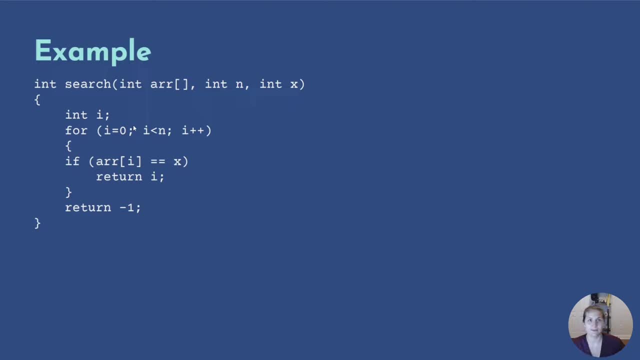 In order to determine the worst case, we must know the case that causes the maximum number of operations to be executed. In this case, let's think what would be the worst case. The worst case would be that x, right here, doesn't exist in the array, So we would just keep going through the array. 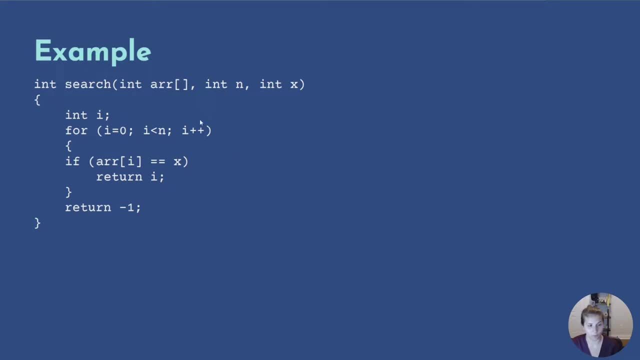 So we would just keep going through the forward loop for the count of n and return negative one. So the worst case in this example is linear time, which would be o n right. So it's basically our big O analysis. Now, before we jump into solving the average case, let's determine what the best case would be for this example. 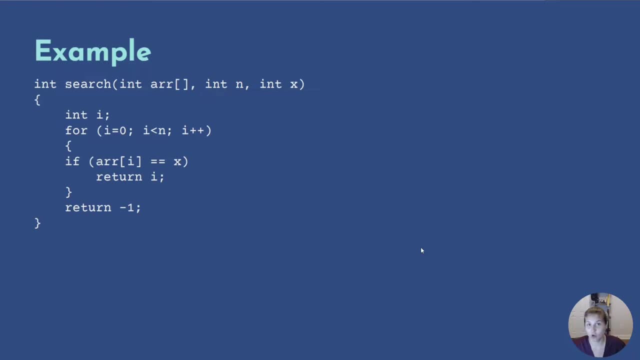 Best case, essentially, is calculating the lower bound of running, of the running time for our algorithm. So in this case, the best case occurs when x is the first item in our array, When x is basically when the array is zero. This would be done in constant time, which would be o one. 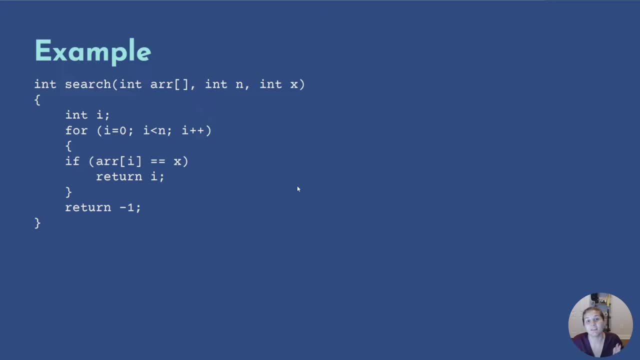 So now it's time to find the average case. In order to find the average case, we need to assume that all the cases- just finding any version of x is uniformly distributed. All possible cases would be n right. So if we're looking for an item, 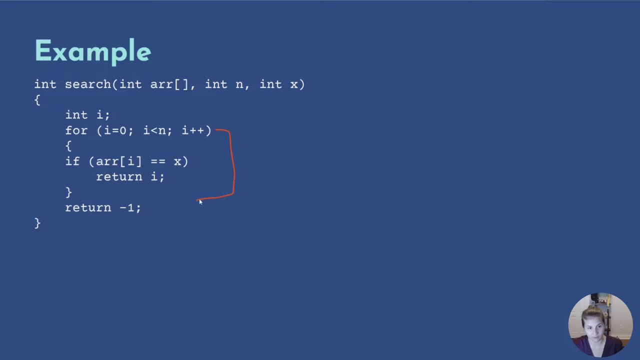 we can go to it potentially here. So inside here we have that dx is greater than or equal to rная. If we look at the other case, we see that here we've got omega positive zero, but it's not at z wherever it stands. So you're simply going to say what's possible if we compare this time with the first. 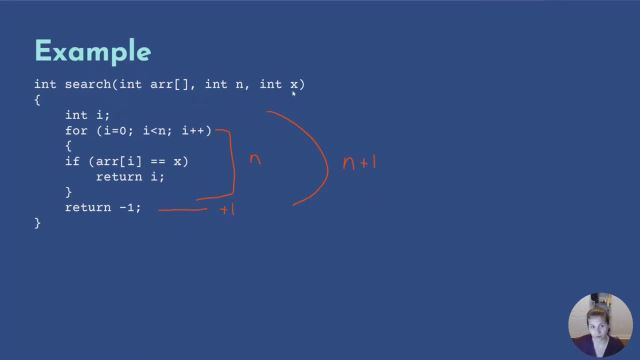 we just have this surrogate starting here and we have vary going on until y is the last. it's going to be uniformly distributed amongst n plus 1.. So the requirement would need to be in the position or it doesn't exist, which means it would be between 1 and n plus 1.. 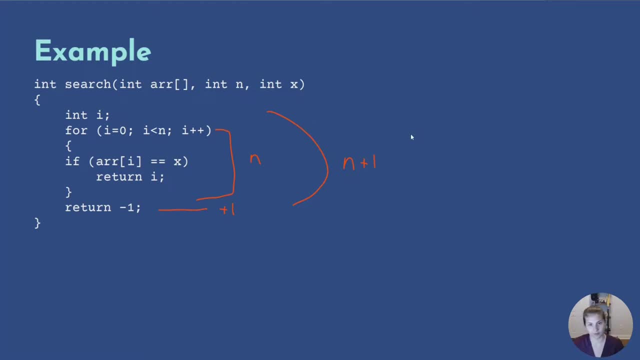 Being uniformly distributed. we're saying that we're finding e of x where we're looking for 1, and 1 could be within the probability of 1 over n plus 1, plus 2 over 1, n plus 1, plus 3, 1 over n plus 1,. 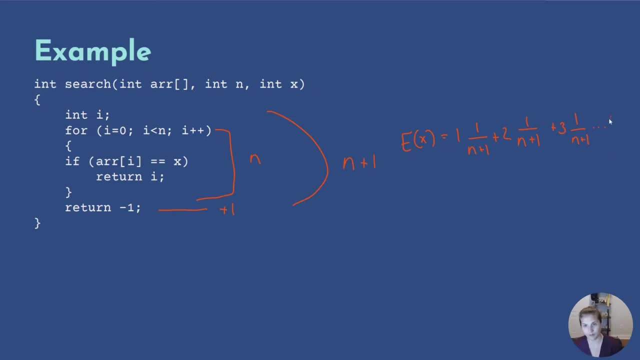 so on and so forth, all the way to n plus 1, which is 1 n times 1.. 1 over n plus 1.. This is our probability. This is the input that we are looking for, This using some fun math. that would be required if you do some calculus. 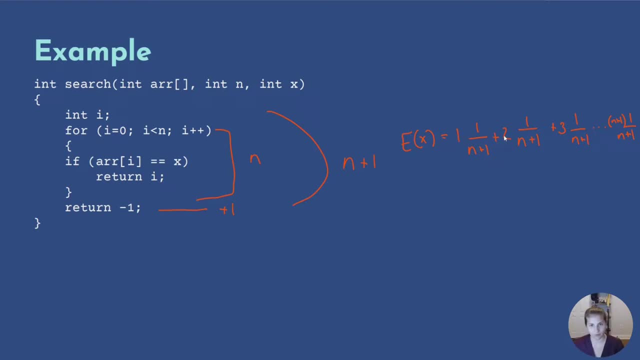 this is our summation, So when we are going through this, we are summing up all the way to n n plus 1.. This can be translated as n plus 1 times n plus 2.. All over 2 n plus 1.. 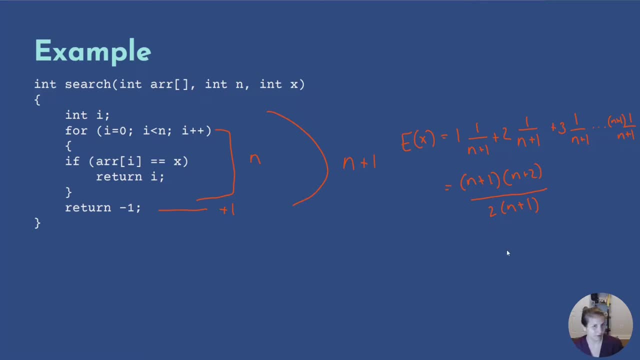 So if we look at this here, we could cancel out our n plus 1.. It's n plus 1.. It's n plus 2 over 2, which translates to an average case of being linear time. This is our average case. 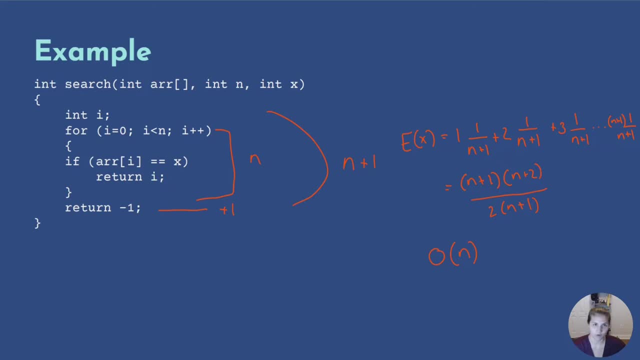 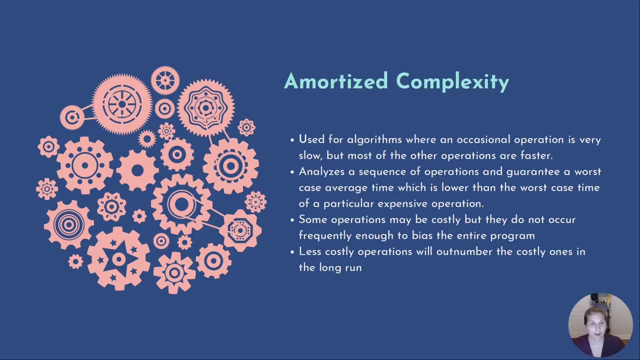 So in this example, our average case and our worst case are actually the same. Now let's talk about another complexity, and that's amortized complexity. Amortized analysis is used for algorithms where an occasional operation is very slow, But for most of the other operations it's faster. 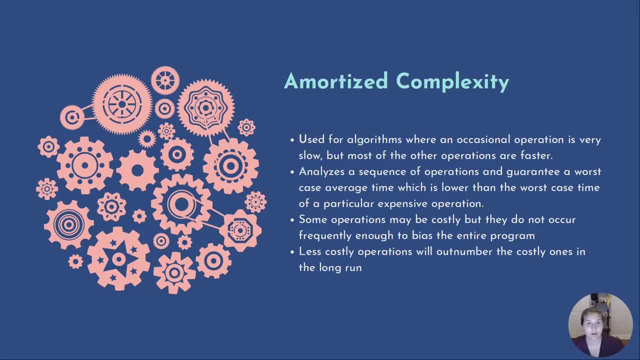 So in this case we analyze a sequence of operations and we need to guarantee a worst case average time Which is lower than the worst case time of an expensive operation. The idea here is that while some operations may be costly, they do not occur frequently enough to bias the entire program. 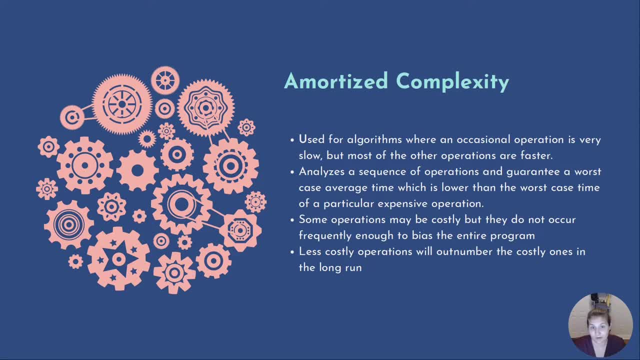 And this is because less costly operations will end up outnumbering the costly ones in the long run, Basically paying back the program over a certain number of iterations. So let's think about this in less abstract. of an example: You make a certain amount a year. 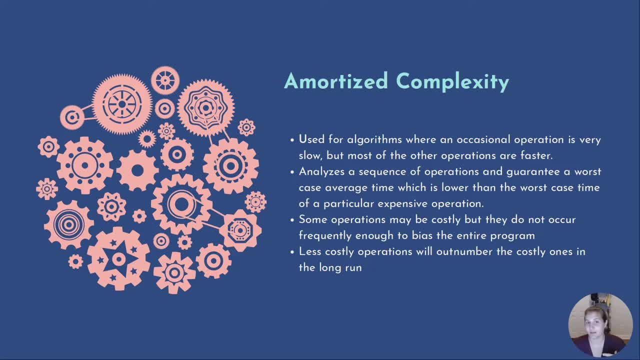 and your monthly expenses need to be less than that amount you make in a year divided by 12.. You can only spend a certain amount of money in a particular month, But if you need to buy a car and that's more than that, 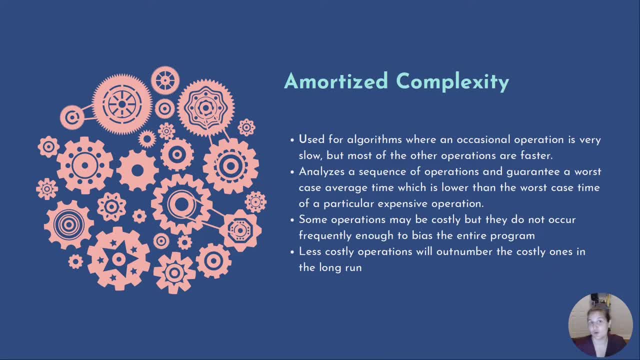 more expensive, then you actually end up offsetting that, because you spend a big amount of money in one month, but in the other months you're going to be saving money for that expensive month. that's what we're doing here: we're saving time with our less costly operations so that we can prepare for a costly operation. 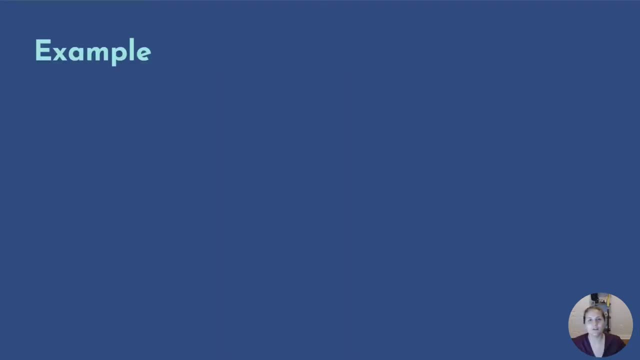 in the long run. so let's think about something in the terms of a table. we want to determine the size of the table. in this example, we're going to do a hash table. there's trade-offs between space and time if we make a hash table really. 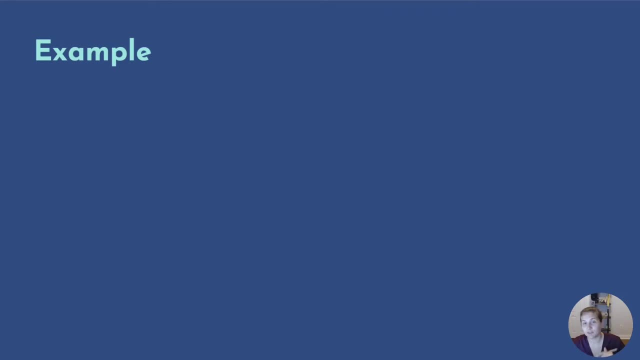 big, the search time becomes fast, but the space required for it is very high. so how do we determine, then, the best size for our table? The solution is to do a dynamic ray application, which means that we double the size of the ray each time it fills up. So what does this mean? 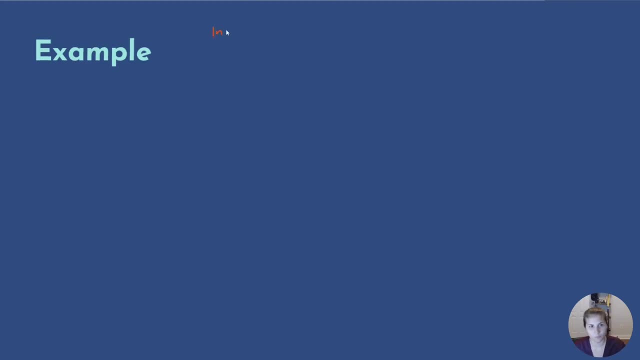 Let's draw it out So: initially our table is empty, which means it has a size of 0. Then we want to insert an item. In this case it's going to be an overflow because our size is zero. So we start off and make our 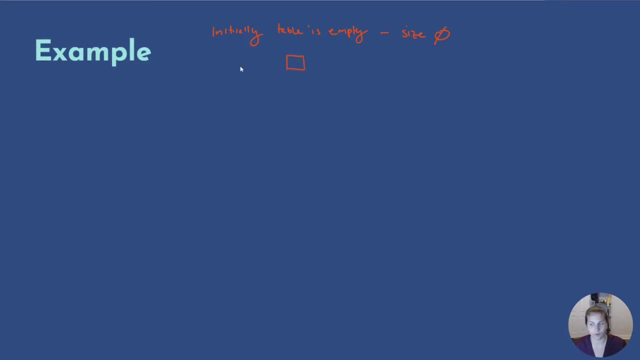 array have one item, We're going to insert one, Then we want to insert two. This is going to cause an overflow again, so So we double our array. So our array is the size of one, So we double it. It now has two. 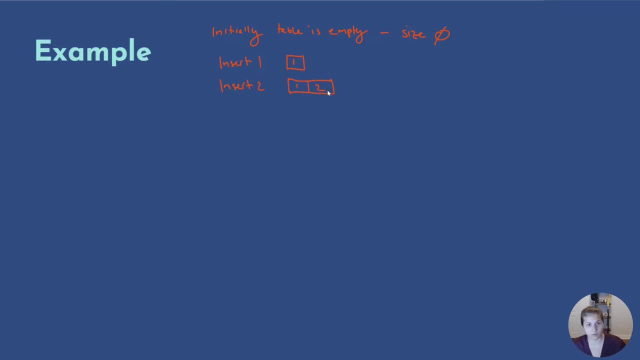 So we have one and two. Now we want to insert three, So we do insert for three. Well, there's an overflow. We're going to double the size. So in this case we have one, two, three and then a free space. 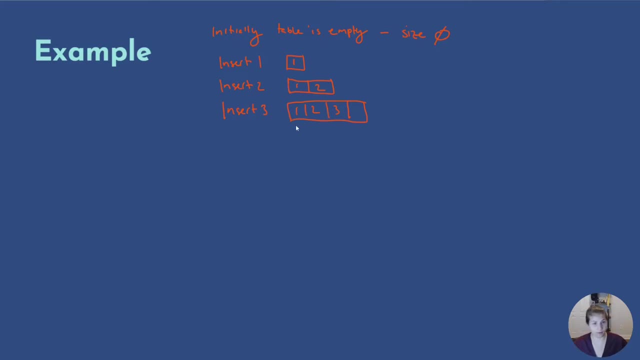 So when we insert four, we will not overflow. So we insert in four. We're going to have space to put four in One: two, three, four. When we want to add five, though, again we get an overflow. 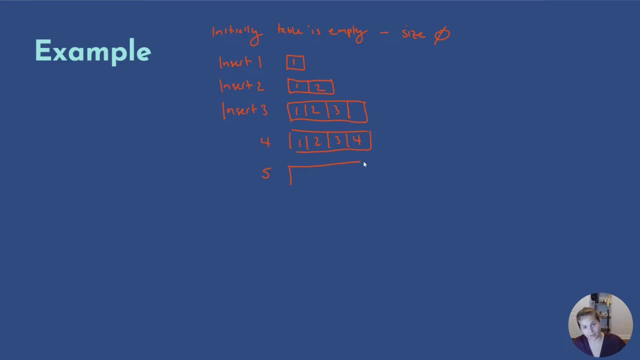 So we double the size of our array. In this case, now it becomes eight, Two, three, four, five. So we can insert in six and then seven, the eight. Our next overflow would end up when we want to insert in nine. 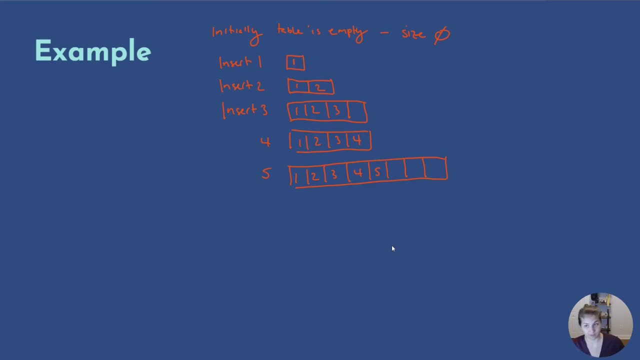 And then we would double the array Two, three, sixteen. So what are the steps that are occurring here? We're allocating memory for a larger table, And this is in the case that the size is going to become twice that of the old table. 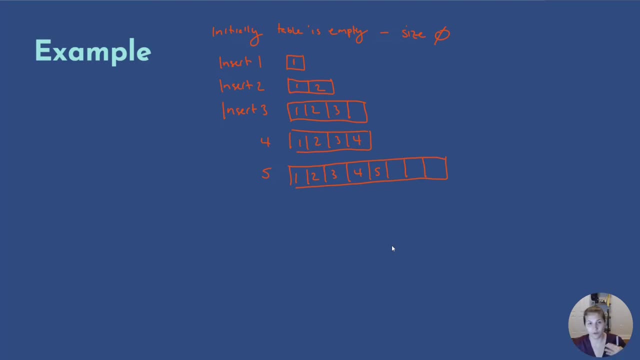 We copy the contents of the old table to the new table And then we free up the old table space. Worst case: an insertion could cost. It could be linear, because we have to copy everything over And then we have to free up the old table space. 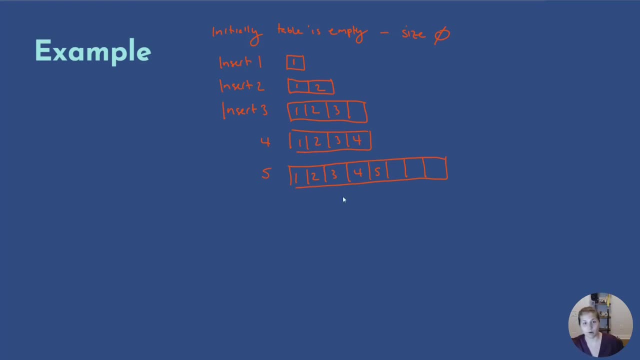 And then we have to free up the old table space And then we have to free up the old table space to the next table. but when we want to insert a new value, like when we insert it in four here, or we insert six, seven and eight, that can be done in constant. 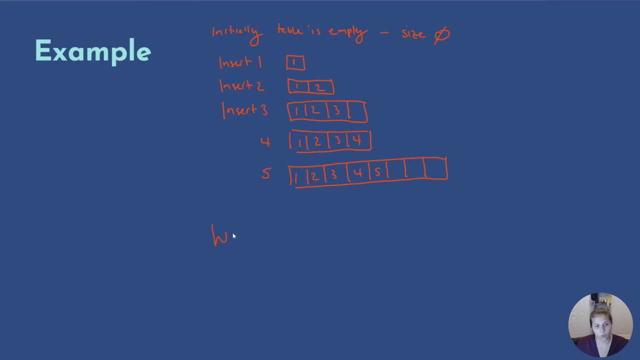 time. so in this example the worst case is o n, but all the remaining insertions done afterwards can be done in constant time, which is o 1, which is our best, as the remaining insertions can be done in this constant time. a sequence of n insertions can always be done in o n time, so therefore n insertions can be. 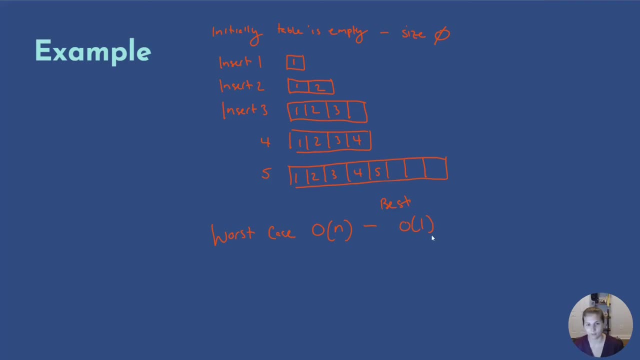 completed in o n time because, worst case, our first one goes o n. all the remaining insertions are going to be o 1 o n plus a bunch of o 1s is still o n. the amortized time is per operation, correct. so amortized time per.